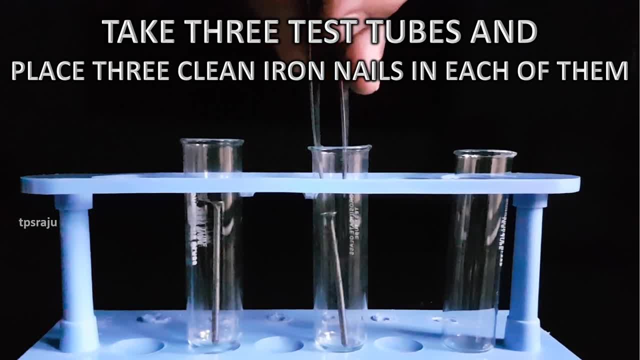 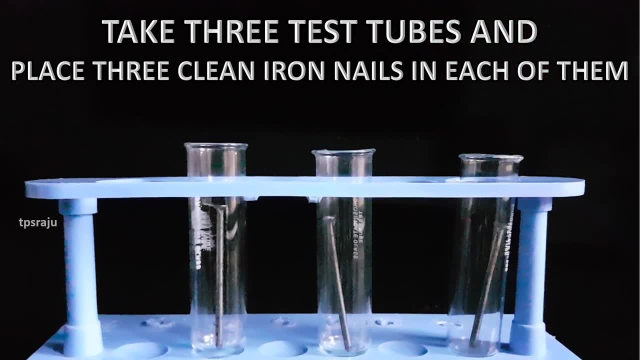 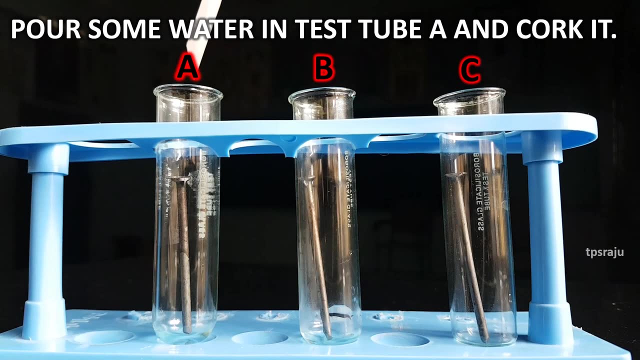 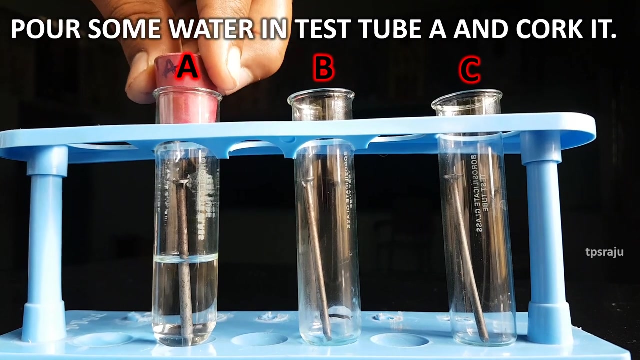 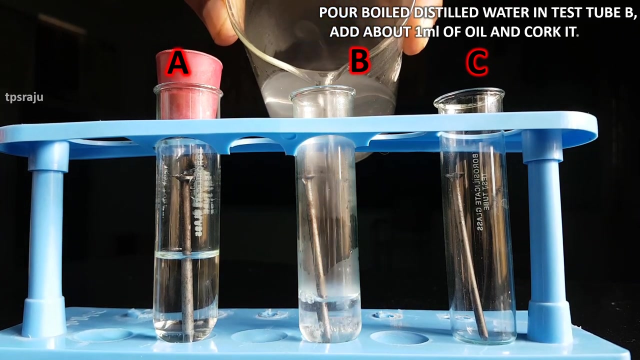 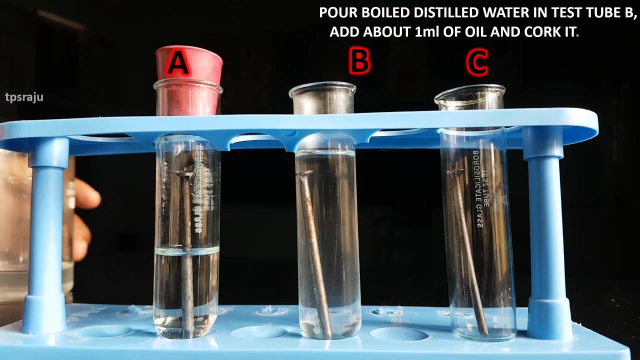 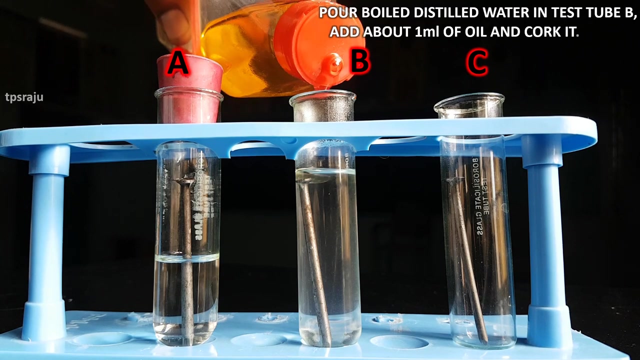 in each of them and label these test tubes A, B and C. Pour some water in test tube A and cork it. Pour boiled distilled water in test tube B, Add about 1 ml of oil and cork it. Put some anhydrous calcium chloride in the test tube. 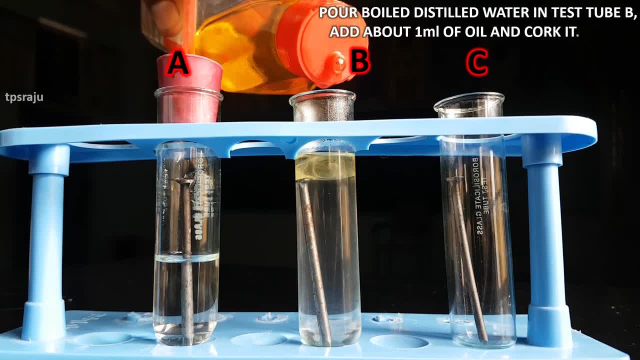 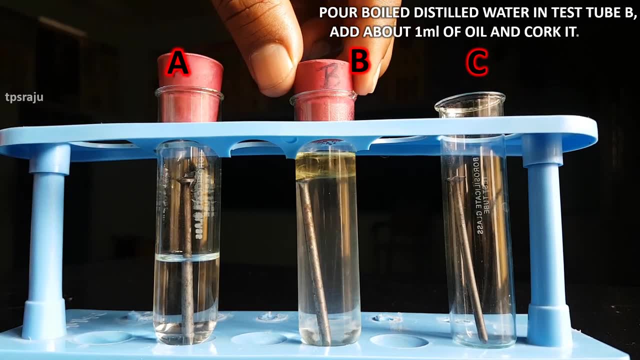 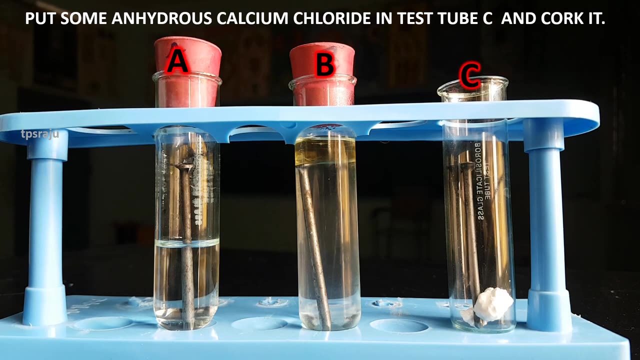 A- Lets put some liquid in the test tube. C. Pourlass on top of air bath. If there is no taka, add hot water. Pile it fast and dry every length of the tube. S— Add about 1 ml of oil and cork it. 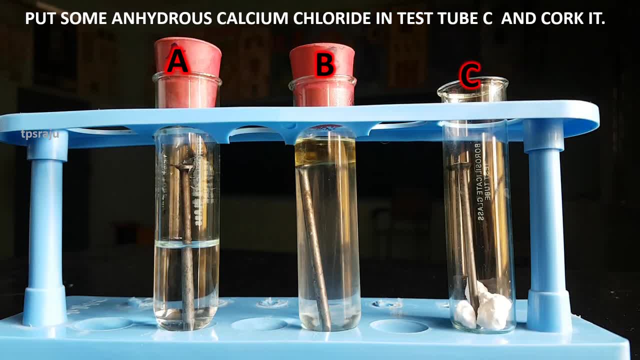 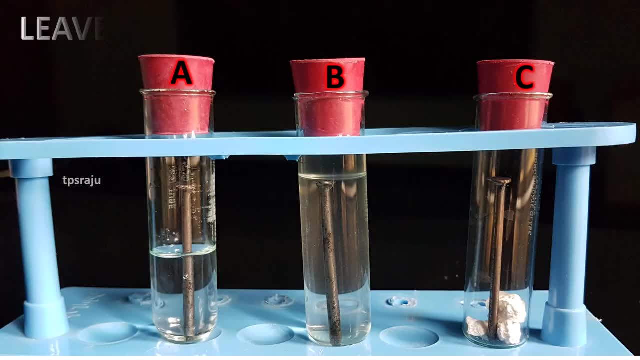 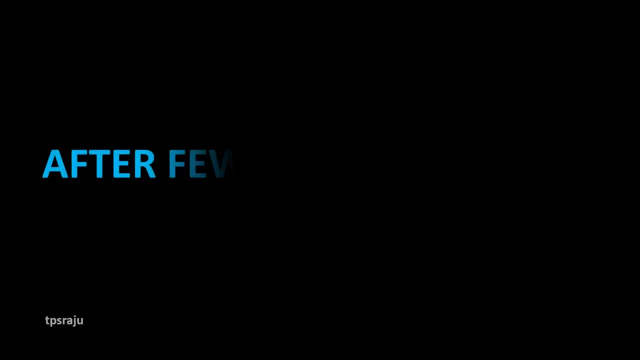 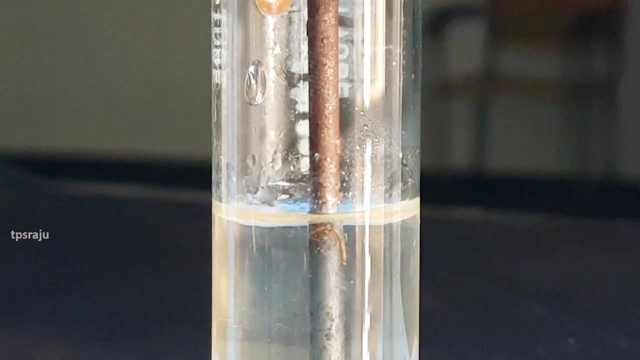 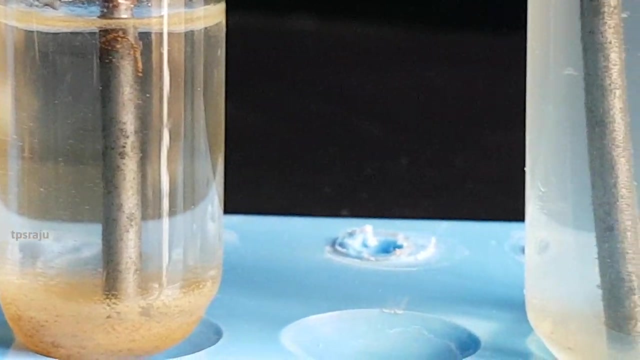 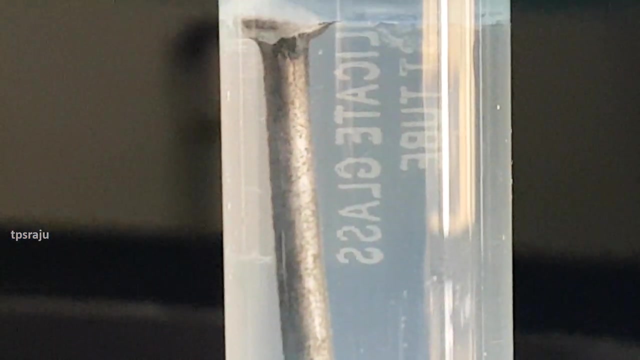 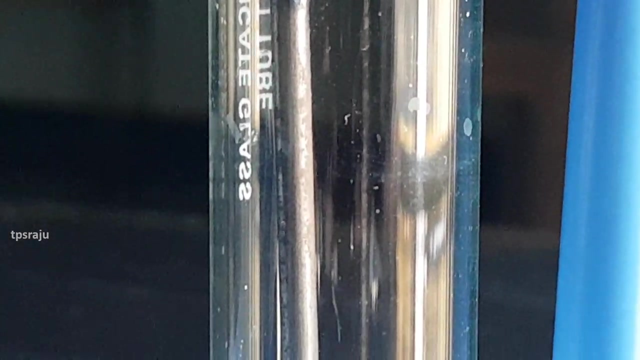 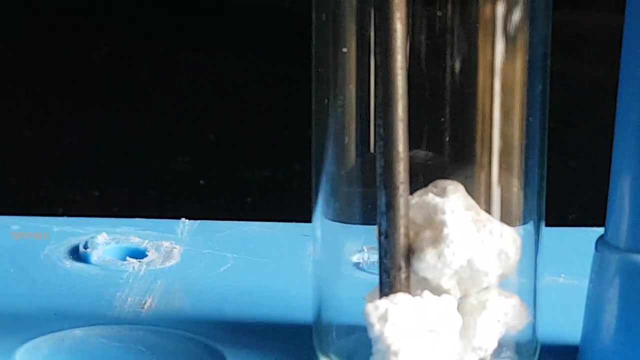 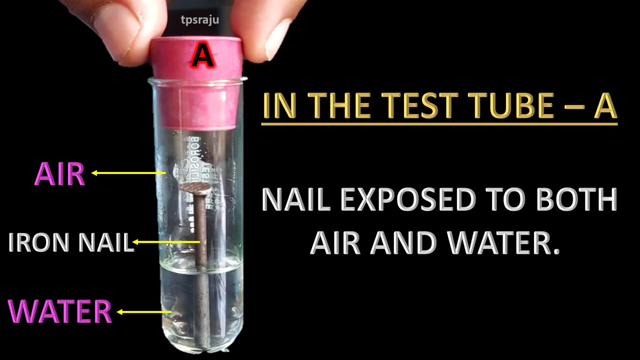 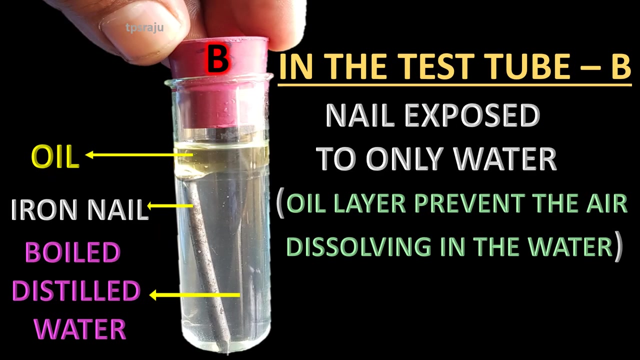 in test tube C and cork it. Leave these test tubes for few days. After few days iron nail can be used to remove rusted in test tube A, But do not rust in test tubes B and C. In the test tube A: nail exposed to both air and water. In the test tube B: nail exposed. 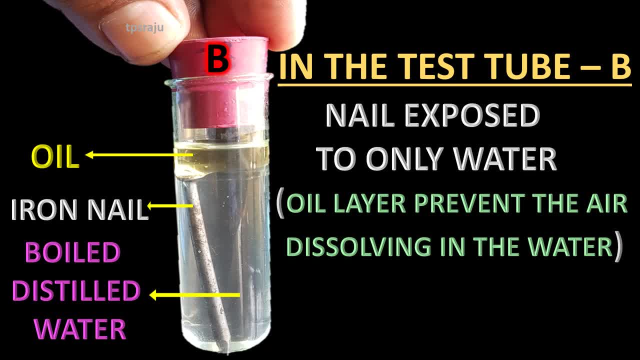 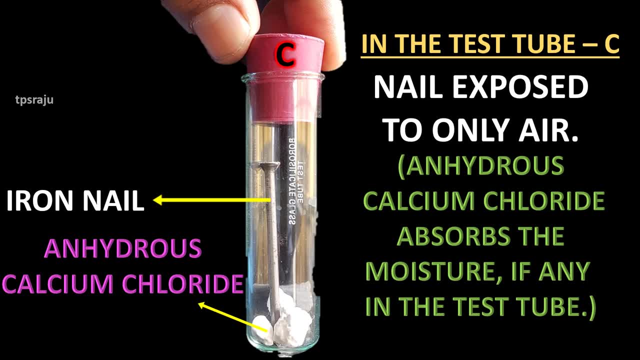 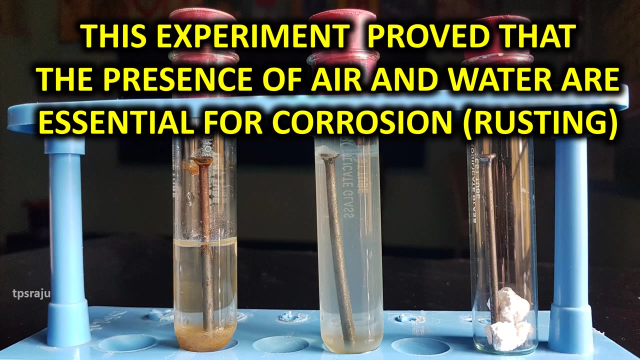 to only water Oil layer prevent the air dissolving in the water In the test tube. C nail exposed to only air, Anhydrous calcium chloride absorbs the moisture, if any, in the test tube. So this experiment proved that the presence of air and water are essential for corrosion.